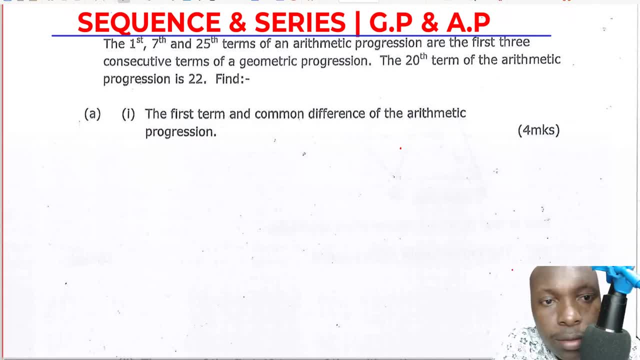 first part. Now we're given that the first, the first, the seventh and the 25th terms of an arithmetic progression are the first three consecutive terms of the geometric progression. So at that point there's something that you need to note: We need to write the first term. 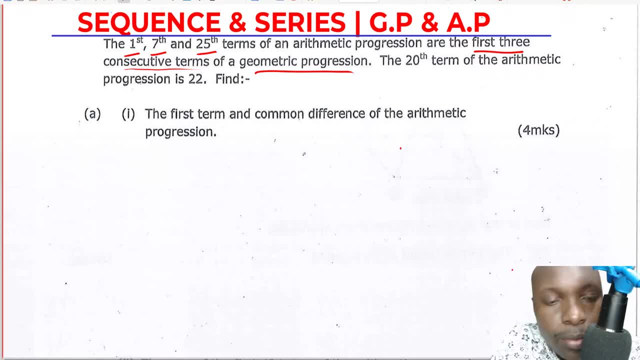 of arithmetic progression. The first term of arithmetic progression is written as A, Then the seventh term is written as A plus 6D. Remember, for an arithmetic progression it has a common difference And that is what gives the difference between a GP and an AP. 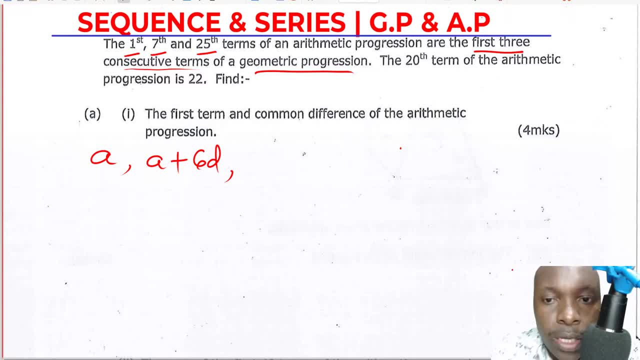 So for a geometric progression it has a common ratio And the nth term of an arithmetic progression is given by A plus n minus 1D, where A is the first term, n is the position of the term, So if it is the first, 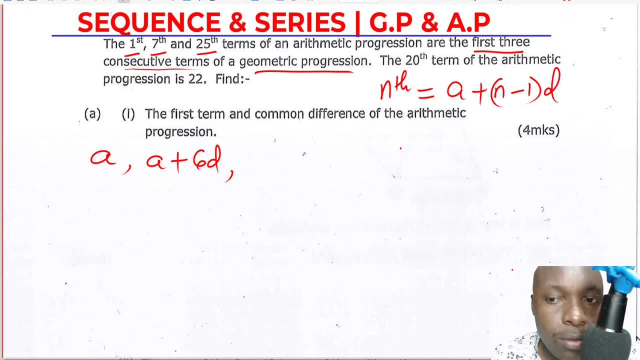 term n will be 1.. If it is the second term, n will be 2.. And then D is a common difference. So when you want to get the seventh term, just come here where you have n and substitute n with 7.. So that is, where you get 7 minus 1,, you get 6D. Then the 25th term will be A plus 24D. 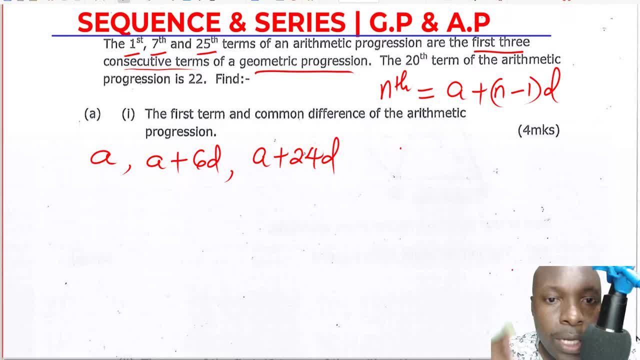 Now, this is the first, seventh and 25th term of the AP. Now we're given that these forms the first three consecutive terms of a GP. So the three of them, the way they are, they form three consecutive consecutive means they follow each other of a GP. And what do you know of a GP? A GP has a common. 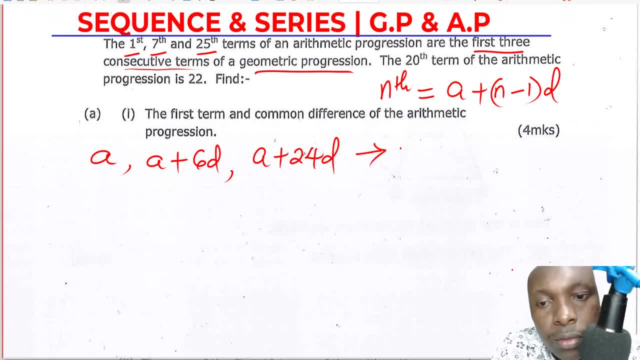 ratio. So if this one forms a GP, the consecutive term, the first consecutive terms of a geometric progression, then this term should have a common ratio. How do we get the common ratio? We take the common ratio will be given by A plus 6D divided by A. That is how we get the common ratio. 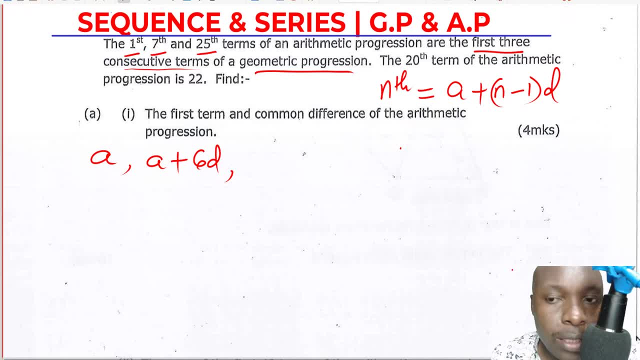 So if it is the first term, n will be 1,, if it is the second term, n will be 2, and then D is the common difference. So when you want to get the seventh term, just come here, where you have n, and substitute n with 7.. 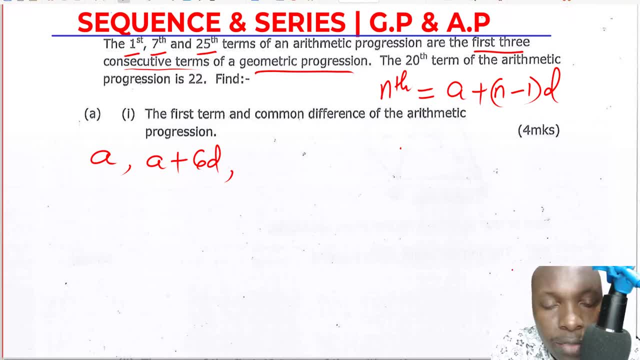 So that is where you get 7 minus 1, you get 6D. Then the twenty-fifth term will be A plus 24D. Now this is the first, seventh and twenty-fifth term of the AP. Now we are given that this forms the first three consecutive terms of a GP. 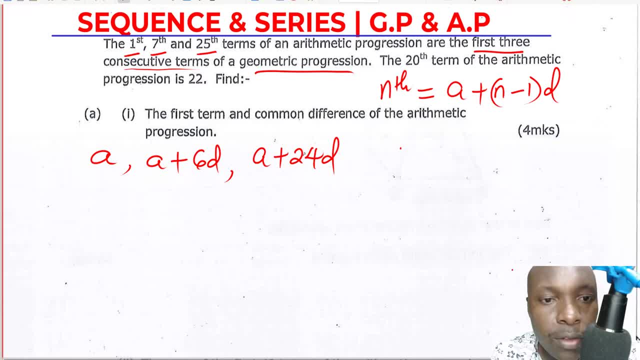 So the three of them, the way they are, they form three consecutive consecutive means, they follow each other of a GP. and what do you know of a GP? A GP has a common ratio. So if this one forms a GP, the consecutive term, the first consecutive terms of a geometric 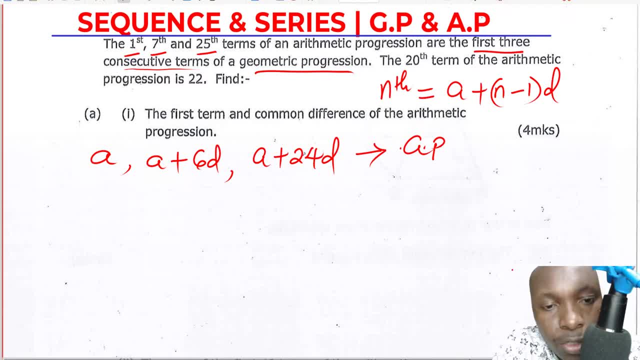 equation, then this term should have a common ratio. How do we get the common ratio? We take the common ratio will be given by A plus 6D divided by A. That is how we get the common ratio And if it is a GP, it should have a common ratio. 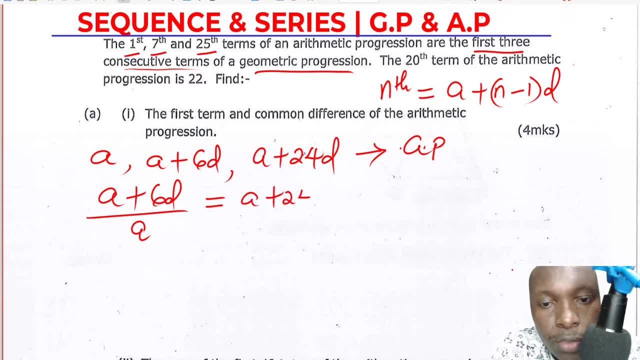 So when I take the other term, that is, A plus 24D divided by A plus 6D, These two should give, Okay, A common ratio. So A plus 6D divided by A is a common ratio. It should be the same with A plus 24D divided by A plus 6D. 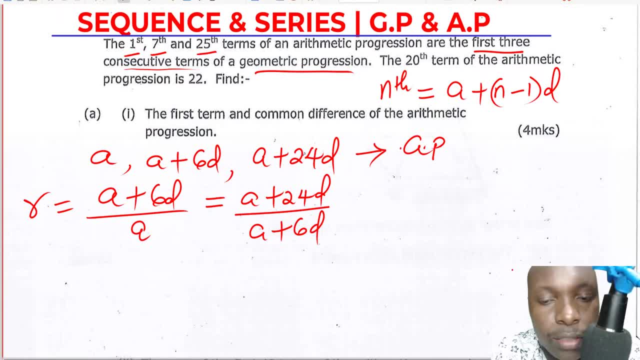 Now having these. now we can work out these and try to multiply out by doing what we call a cross multiplication. It's like this: So I will cross multiply and try to simplify. So these will be A plus 6D multiplied by A plus 6D is equal to A. This is A plus 24D. 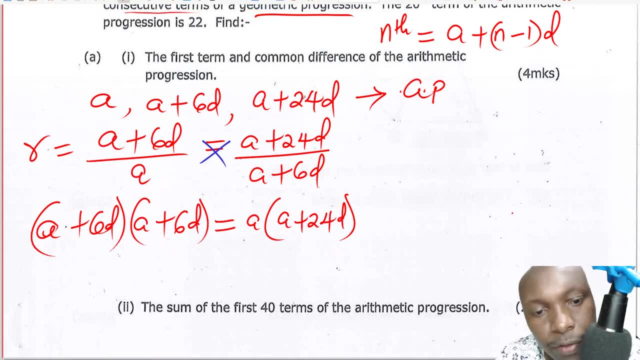 So cross multiplying. We don't know whether this space will be enough, So to simplify this one, When you multiply A plus 6D, Multiplied by A plus 24D, Multiplied by A plus 6D, Let me try to save this space here. 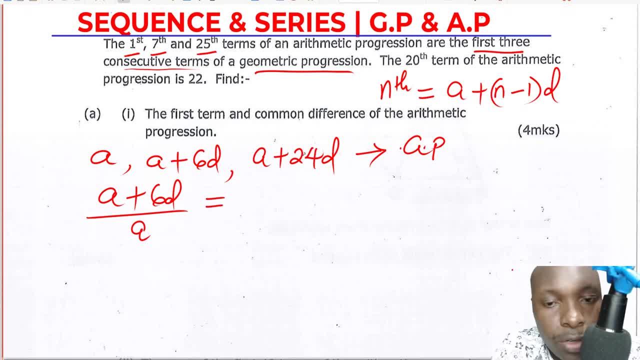 And if it is a GP it should have a common ratio. So when I take the other term, that is, A plus 24D divided by A plus 6D, these two should give a common ratio. So A plus 6D divided by A is the common ratio. it should be the same with. 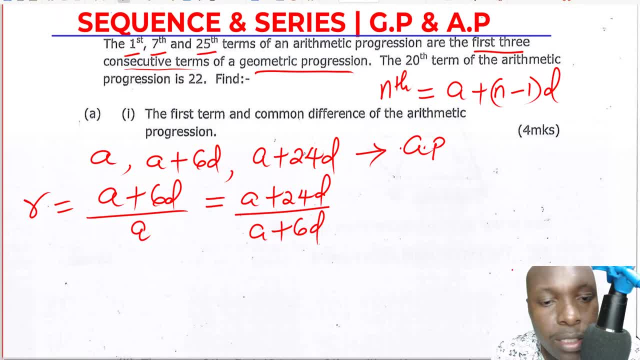 A plus 24D divided by A plus 6D. Now having these, now we can work out these and try to multiply out by doing what we call a cross multiplication. It's like this: So I will cross, multiply and try to simplify. So these will be: 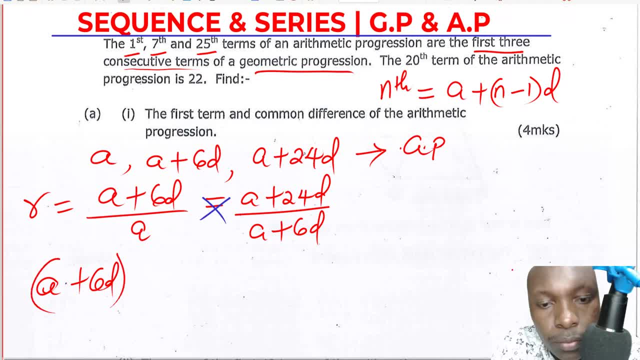 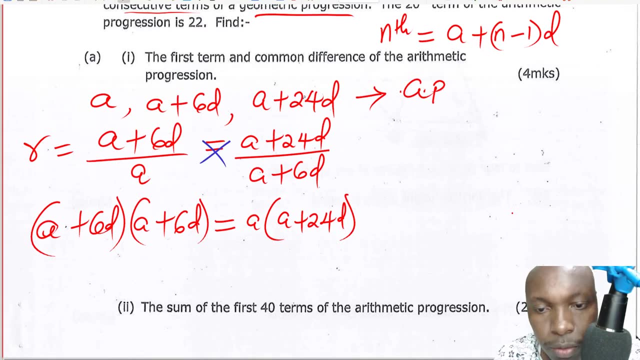 plus 6d. multiply by a plus 6d is equals to a. this is a plus 24d, so i'm cross multiplying. i don't know whether this space will be enough, so to simplify this one, uh, when you multiply a plus 6d, multiply by a plus 6d. let me try to save this space here. now you know how. you know how to expand. 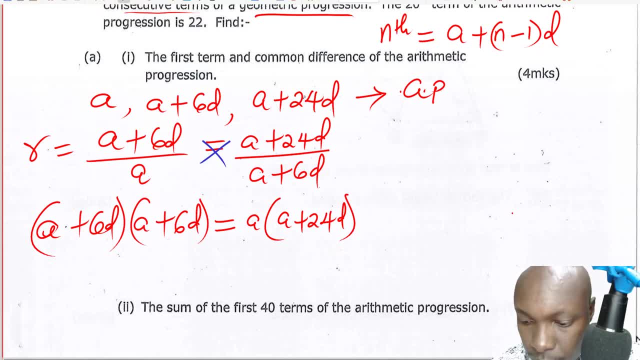 this. so when you expand this because of space, uh, there's something that you need to get here. this will give a squared, a squared plus. this will be 12 a d plus 36 d squared. that is what you get when you expand: a plus 6d a plus. multiply by a plus 6d a squared. 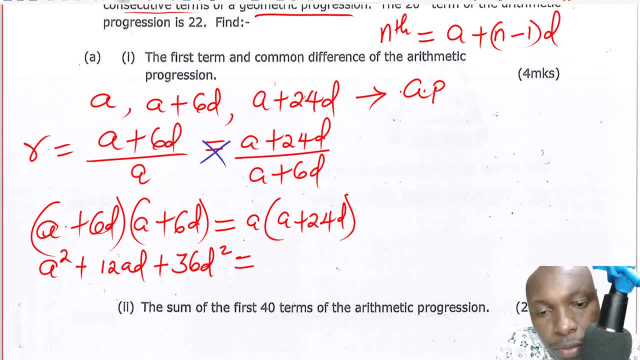 plus 12 a d plus 36 d squared, then this one should be equal to. this is a squared plus 24 a d. so that is what you get now from there. you can try to simplify these. you can see we have a squared there and a squared there, so that when you 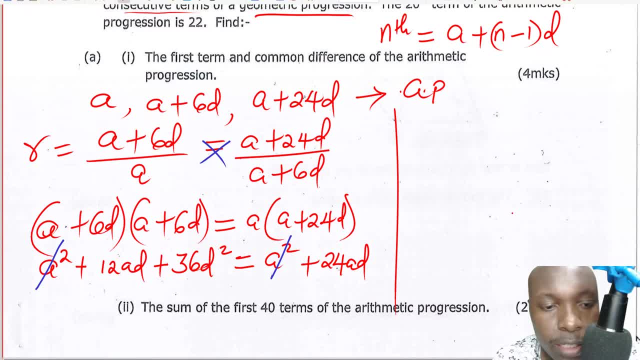 you bring them to one side, they don't get subtracted and a squared will be subtracted and you'll have it at the end at that point, so that one is gone. so now you have- uh, you can take this one to the other side so that you have. 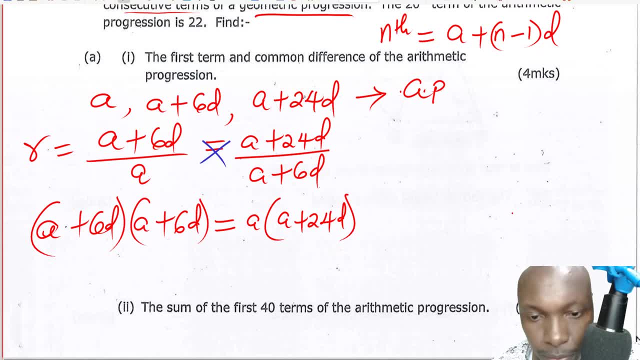 Now you know how to expand this, So where do you expand this one? Because of space, There is something that you need to get here. This one will give A squared, A squared plus. This will be 12AD plus 36D squared. 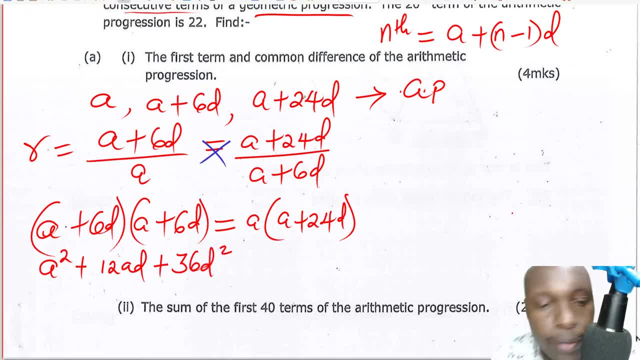 Okay, Okay, Okay. That is what you get. when you expand A plus 6D, Then this one should be equal to. this is A squared plus 24AD. So that is what you get Now from there. we can try to simplify these. 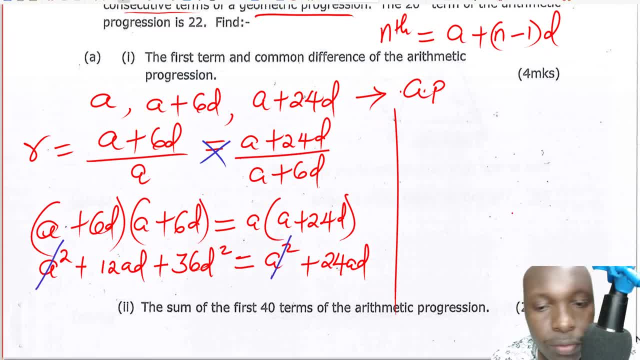 You can see we have A squared there and A squared there, so that one, If you bring them to one side, they don't get subtracted, and a squared will be subtracted and you'll have it the end at that point, so that one is gone. so now you have- uh, you can take this one to the other side so that you 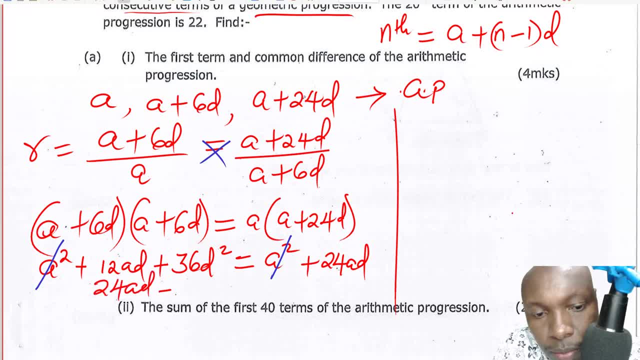 have 24 ad minus 12 ad and then minus 36, d squared is equals to zero. you're just trying to take everything from the left hand side to the right hand side and this one will give the work of these 24 ad minus 12 ad. we get 12 ad minus 36. 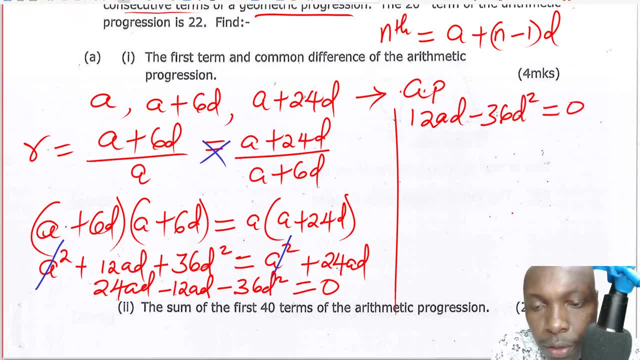 d squared is equals to zero. so what is common here? uh, you can see that um 12, 12, d is common. so you have, uh, we have a. so when you factor out, you have a subtract um, this would be: 3d is equals to zero. so from this point, uh, you get 12, d is equals to zero. 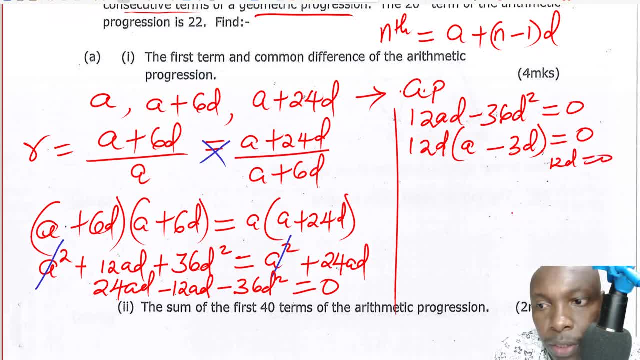 and the one that will be very important, that will help us to work out, is this part here: when you're multiplying two numbers and the solution is zero, that is a 12 d multiplied by a minus 3d. it is either 12 d is equals to zero or 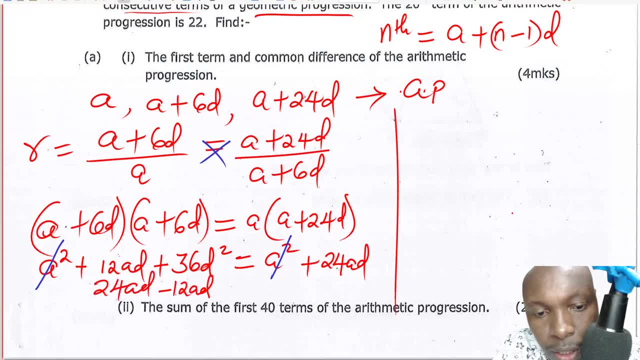 24 a d minus 12 a d, and then um minus 36 d, squared is equals to zero. you're just trying to take everything from the left hand side to the right hand side and this one will give um the work of these. 24 a d minus 12 a d, we get 12 a d minus 36 d. squared is equals to zero. 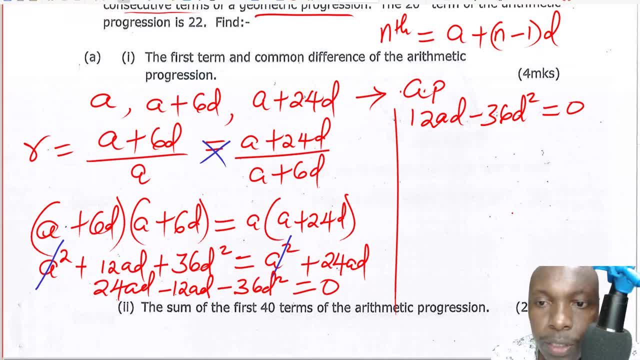 so what is common here? uh, you can see that, um 12, 12d is common. so you have, we have a. so when you forget out, you have a subtract, um, this will be 3d is equals to 0.. so from this point, uh, you get, 12d is equals to 0. 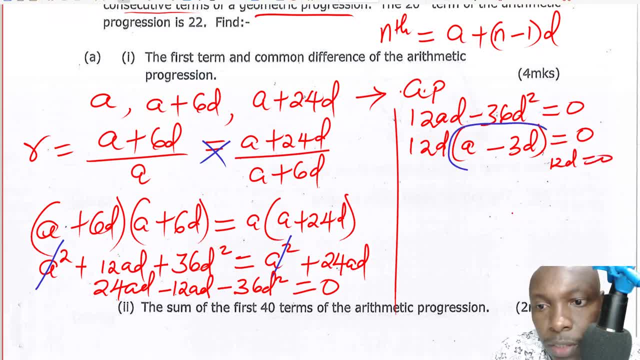 and the one that will be very important, that will help us to work out, is this part: here: when you multiply two numbers in the series, solution is zero. that is a 12d multiplied by a minus 3d. it is either 12d is equal to zero or 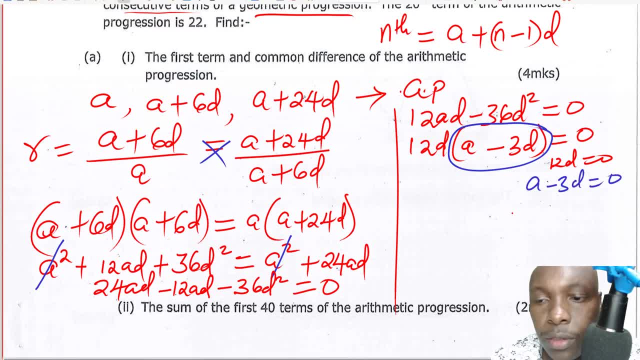 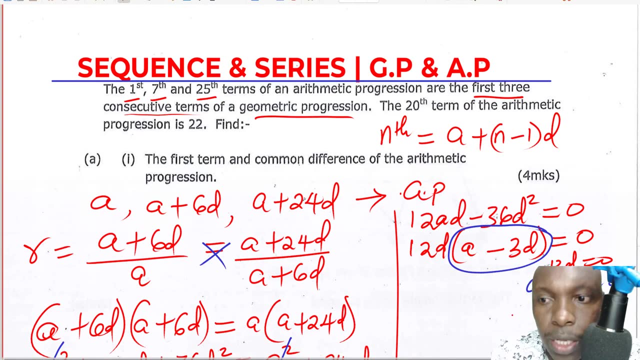 a minus 3d is equal to zero, and if this is the case, you get a is equal to 3d. now, at that point, now, we should be good position to proceed. the next statement, something else that we're given here. the 20th term of the arithmetic progression is 22 20th. 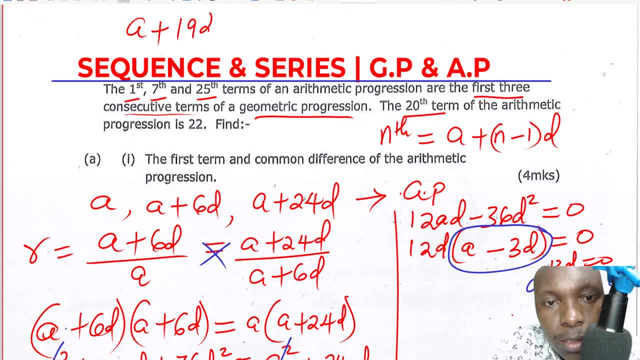 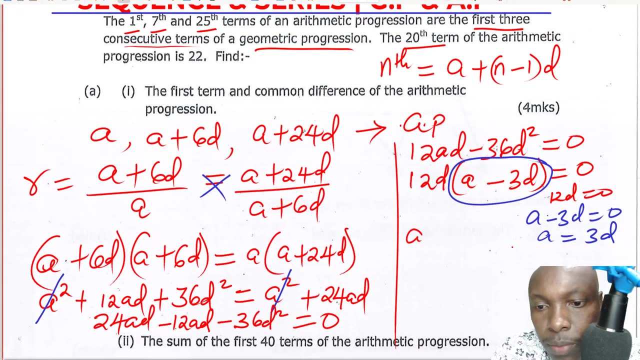 term is written as a plus 19d and they're only given to be 22. so the 20th term, a plus 19d, is equal to 22. so having that now, we should be in a position to work it out. so a plus. 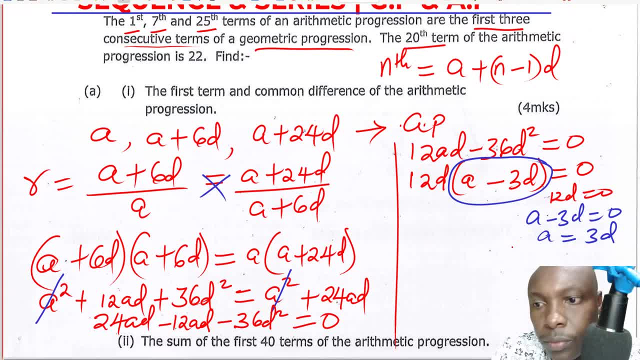 a plus, a plus, so a plus 19d is equal to 22 and having these and these, we should be able to work out so this multi-insecution. so let me just use substitution a is 3d, so substituting the zone, the zone a is 3d. 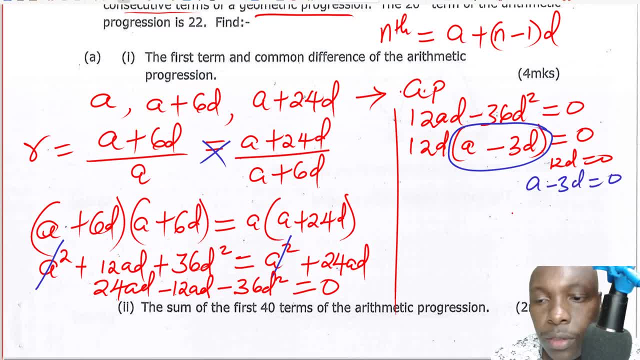 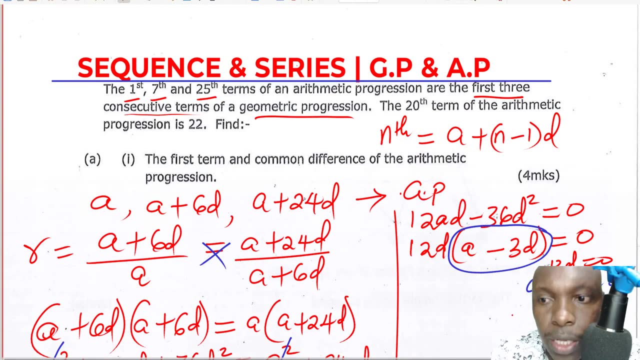 a minus 3d is equals to zero, and if this is the case, you get a is equals to 3d. now, at that point, now, we should be good position to proceed. the next statement, something else that we're given here: the 20th term. 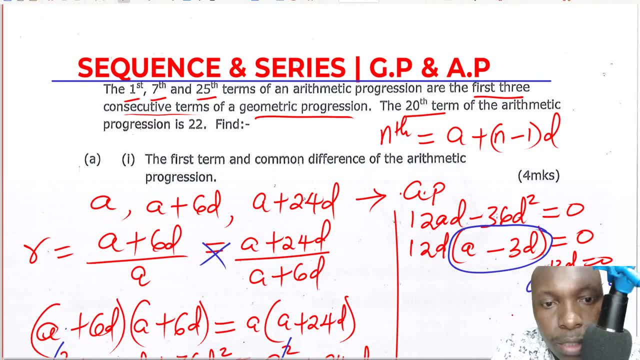 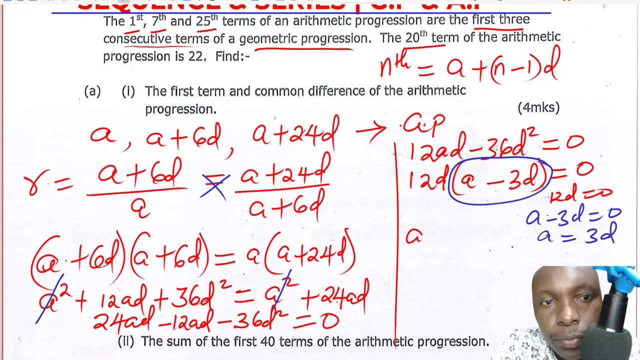 of the arithmetic progression is is 22.. 20th term is written as a plus 19 d, and they're only given to be 22, so the 20th term, a plus 19 d, is equals 22.. so having that- and now we should be in a position to work it out- so a plus. 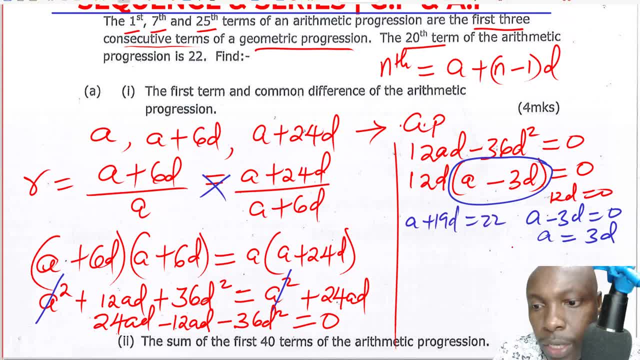 so a plus 19d is equals 22.. and having these and these we should be able to work out. so this is a multi-inheritance equation. so let me just use substitution A is 3D, so substituting the zone, the zone A is 3D. 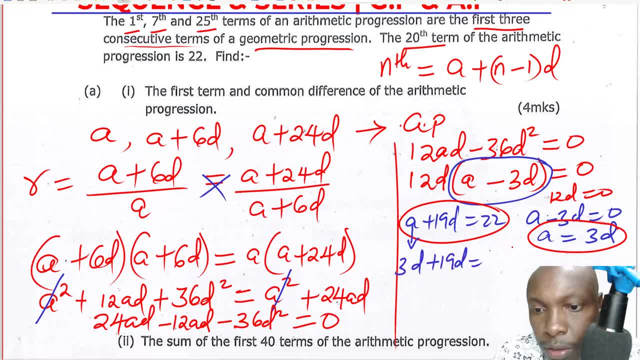 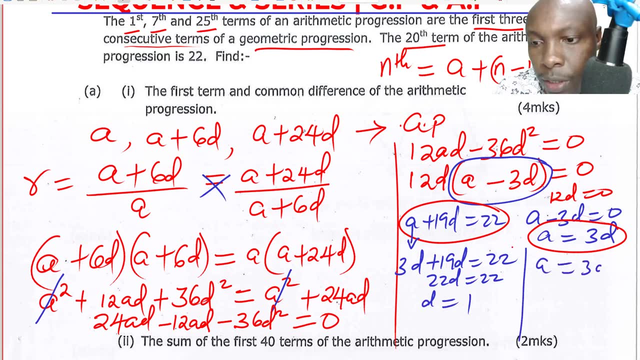 plus 19D is equal to 22, so this will give 3 plus 19. you get 22D is equal to 22, so D is equal to 1, and since we have A is 3D, so A will be. D is 1, so A will be 3. 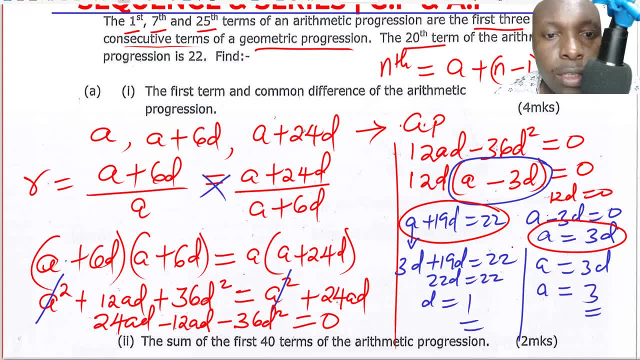 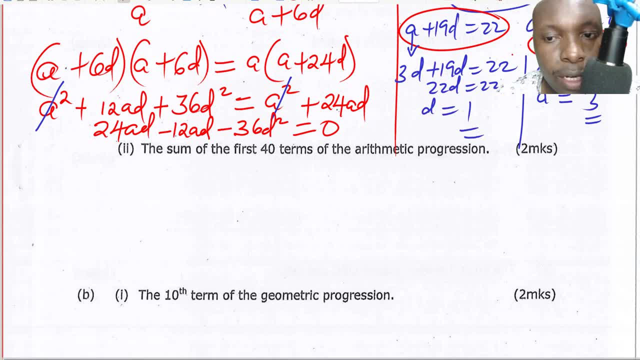 so we found the first term and the common difference of the arithmetic progression. now the second part, the sum of the first 40 terms of the arithmetic progression, sum of the first 40 terms. so this question: you need to know how to get the sum of a number of terms of any arithmetic progression. 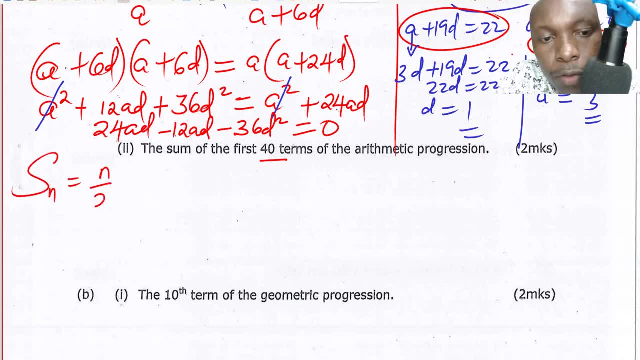 just give it given by n over 2, then 2a plus n minus 1, led by the common difference. so this is how we get the sum of any number of terms that are given of any any arithmetic progression. so substituting 40 terms, so n will be 40. 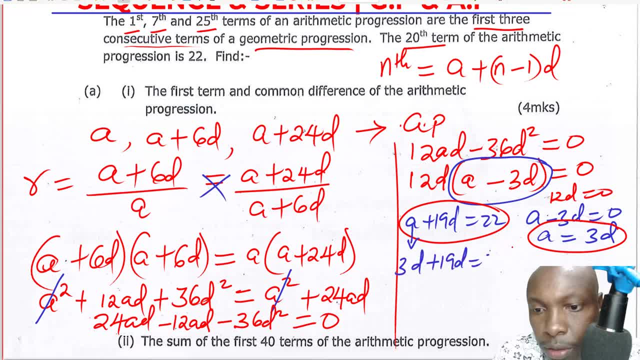 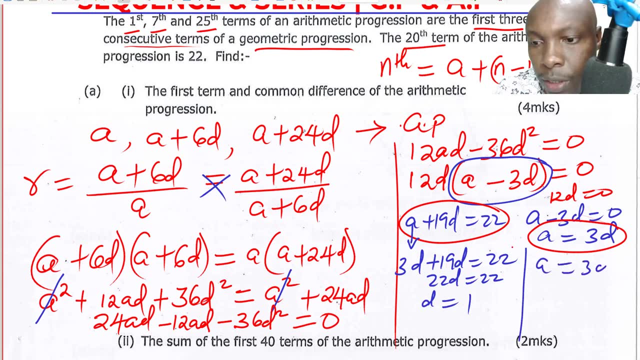 plus 19d is equal to 22. so this will give um 3 plus 19. you get 22d is equal to 22, 22, so d is equal to 1 and um. since you have a is 3d, so a will be, d is on, so it will be 3. 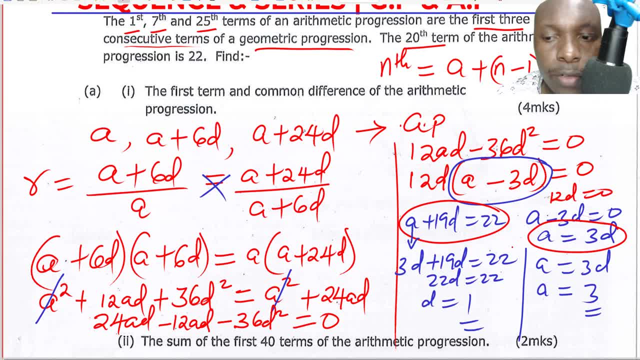 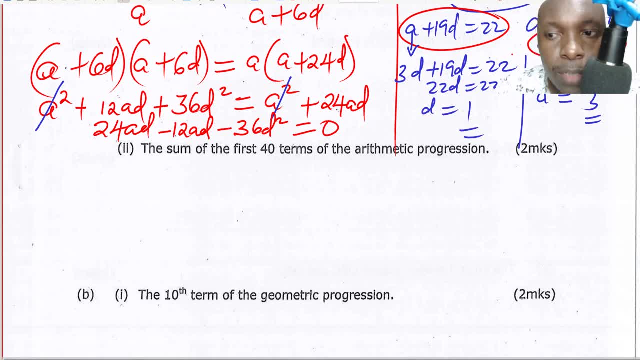 so we found the first term and the common difference of the arithmetic progression. now the second part, the sum of the first 40 terms of the arithmetic progression, some of the first 40 times. so to solve this question, you to know how to get the sum of a. 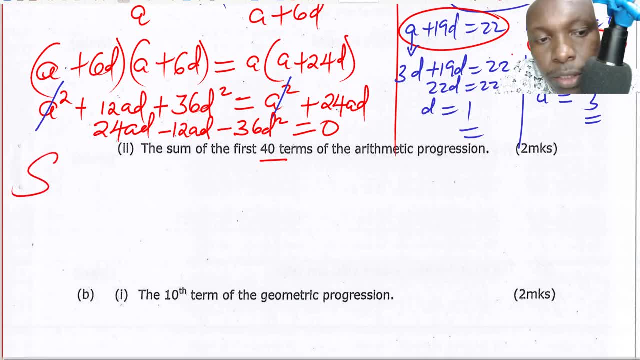 number terms of any arithmetic progression. it is given by n over 2, then 2a plus n minus 1, led by the common difference. so this is how we get the sum of any number of terms that are given of any any arithmetic progression. so substituting 40 terms, so n will be 40. 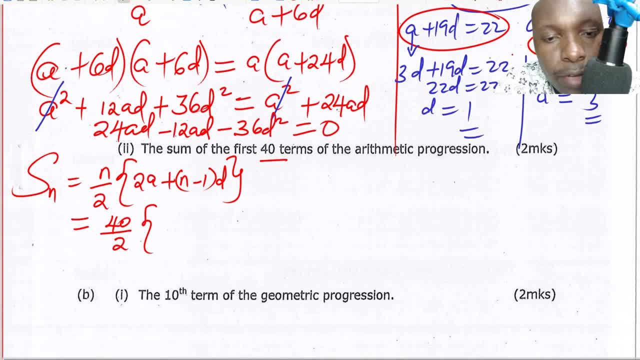 we already have a. a is a 3, so this will be 2 times 3, which will give 6. then n again is 40, so this is a 40 minus 1. you get 39 d like that. so this will give 20 multiplied by 6 plus. 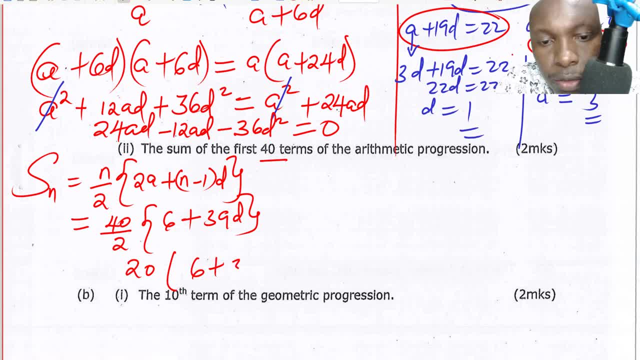 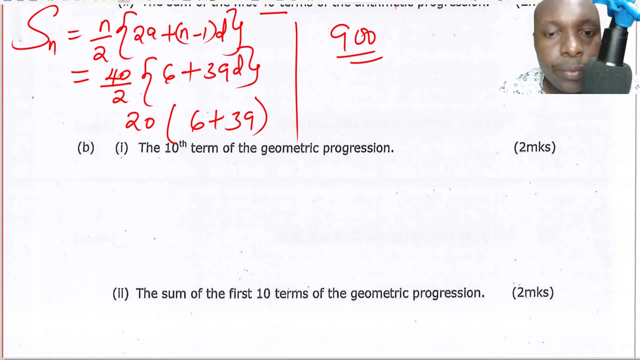 then 39 times d, d is 1, so this will be 39. working out this using a calculator, are you get this- would be 900. so the sum of the first 40 terms of arithmetic progression will be 900. now the 10th term of the geometric progression. so to read the 10th term, how do you write the? 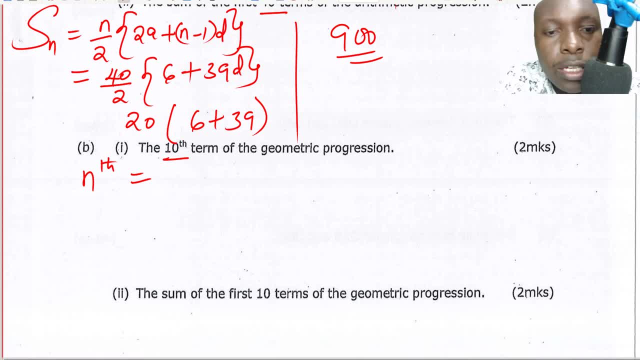 nth term of any of a geometric progression. nth term of a geometric progression is given by a. r is my power, n minus 1. a r is for n minus 1, where a is the first term, r is the common ratio, n is the position of the term. so in this case it's 10th term, n will be 9. 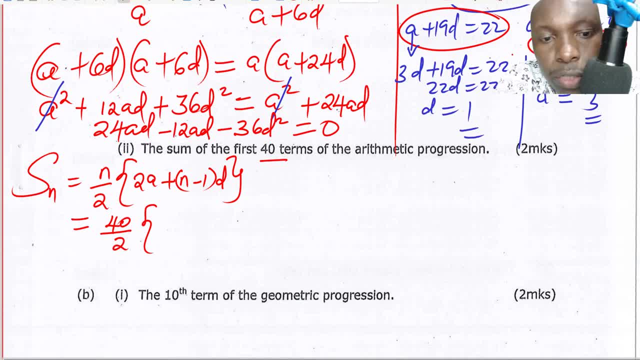 we already have A. A is 3, so this will be 2 times 3, which will give 6. then n again is 40, so this is 40 minus 1. you get 39 D like that. so this will give 20 multiplied by 6. 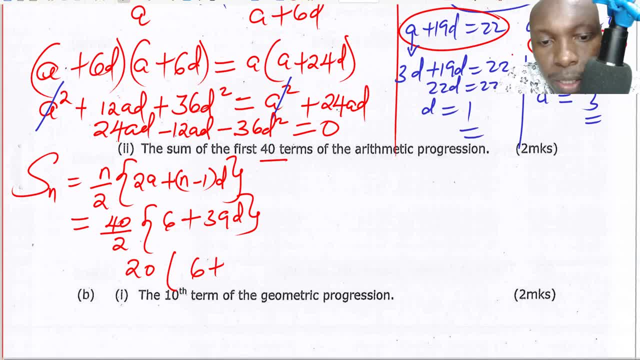 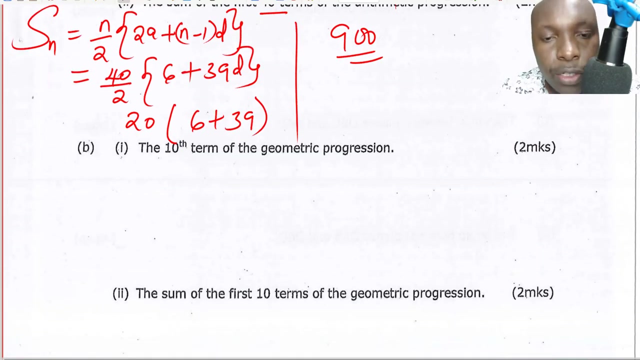 plus then 39 times D, D is 1, so this will be 39. working out this using a calculator, you get this will be 900. so the sum of the first 40 terms of arithmetic progression will be 900. now the 10th term of the geometric progression. 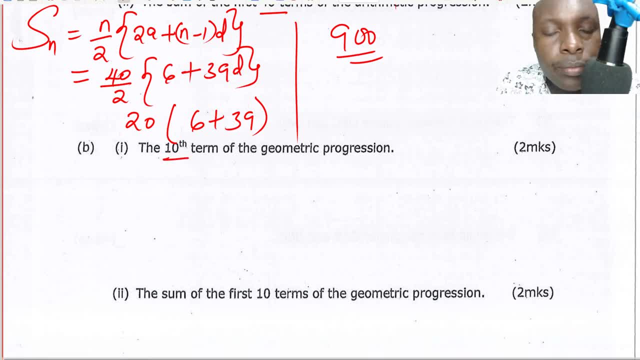 so to read the 10th term, how do you write the nth term of any of a geometric progression? the nth term of a geometric progression is given by Ar raised to the power of n minus 1. Ar raised to the power of n minus 1. 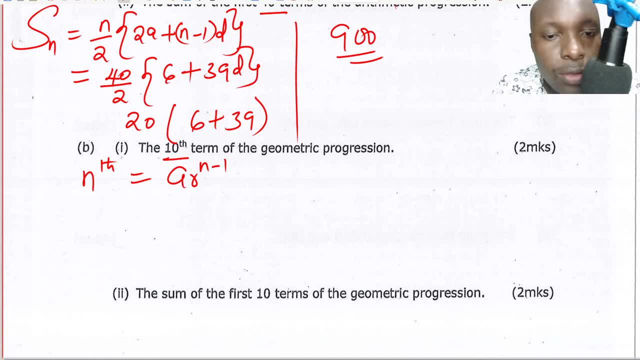 where A is the first term, R is the common ratio, n is the opposition of the term, so in this case it's the 10th term. n will be 9. now the 10th term, the n will be 10. sorry, so if it is the 10th term, 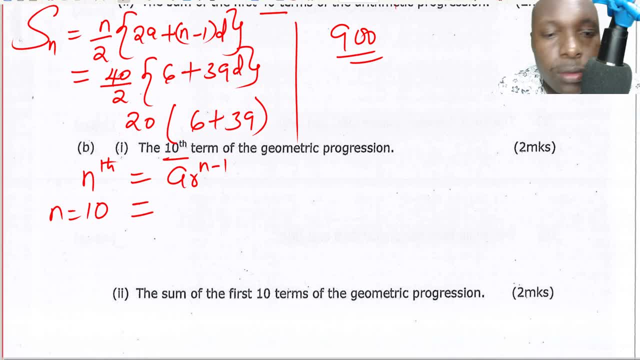 the GP n will be 10, so substituting: here you have A, we already have A. A is the first term we got it as of this. GP is 3, remember that A is 3, and so if you substitute A is equal to substitute A is equal to. 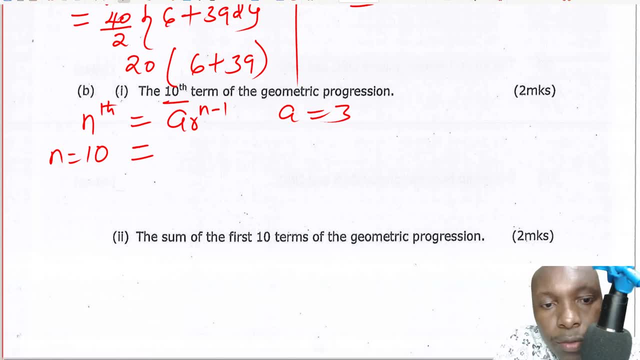 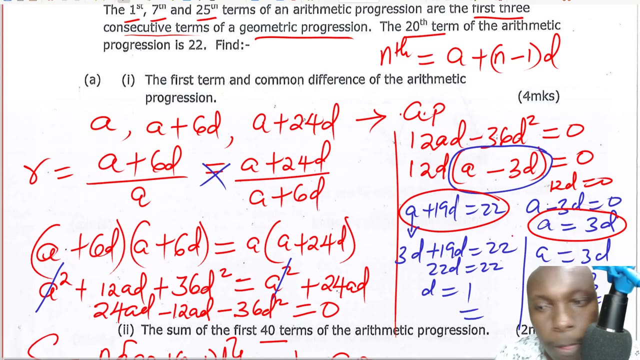 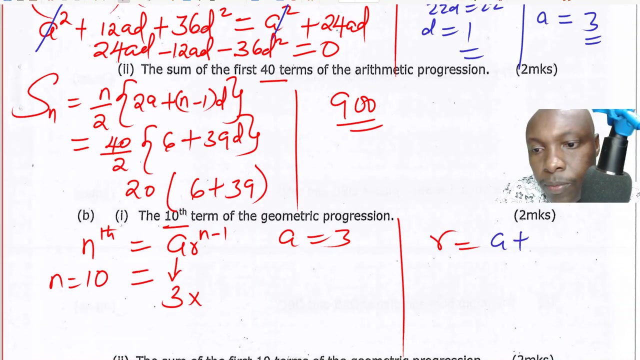 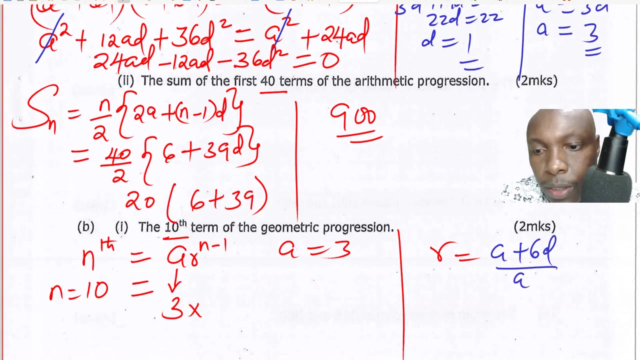 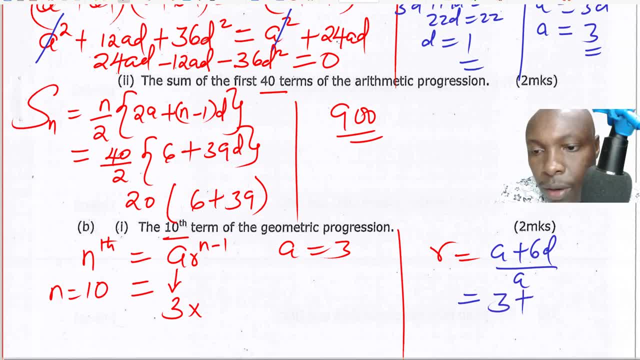 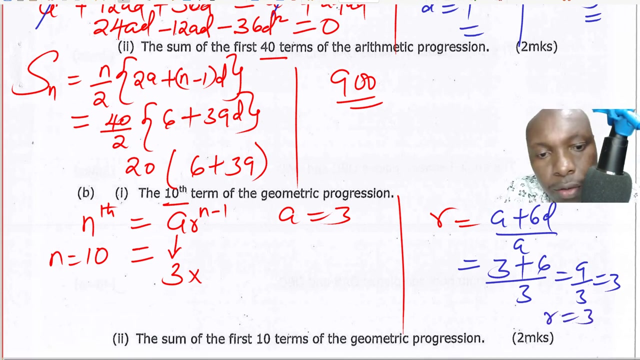 a is 3, then d is 1, and then like that. so this will give 9 divided by 3. so the common ratio is: let me do it again: this is 3 plus. yes, it is ok, it is ok. r is 3. so now substituting here: a is 3. 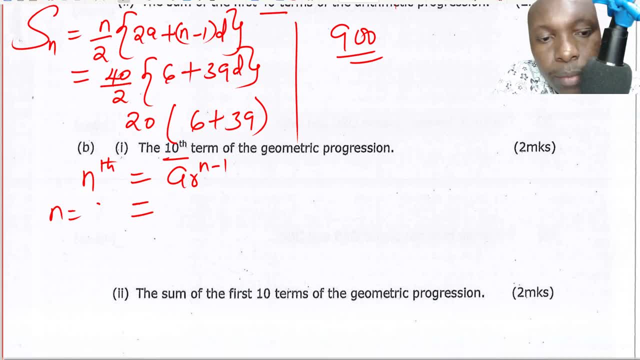 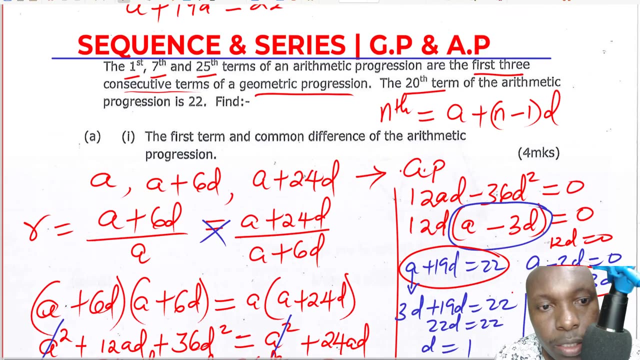 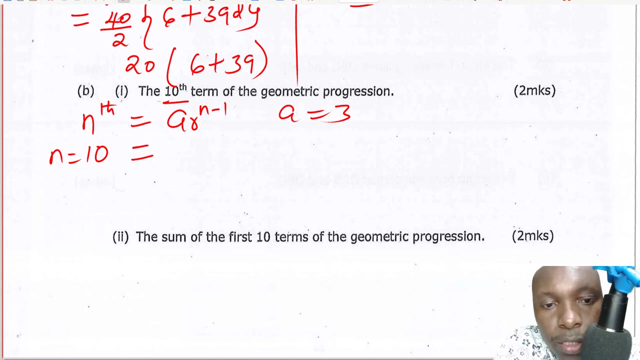 now the 10th term, the n will be 10. sorry, so if it is the 10th term, the gp n will be 10. so substituting: here: you have a. we already have a, a. a a is the first time we got it as of this gp is 3, remember that a is 3, and so you substitute a is. 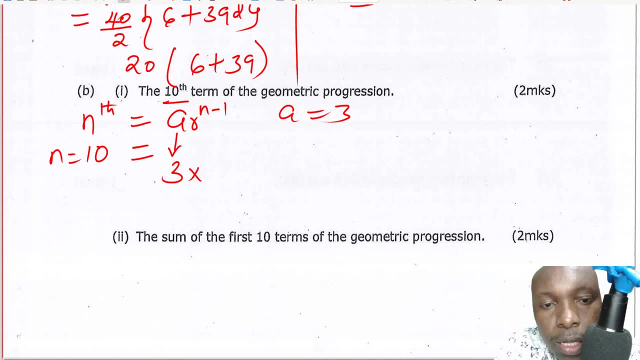 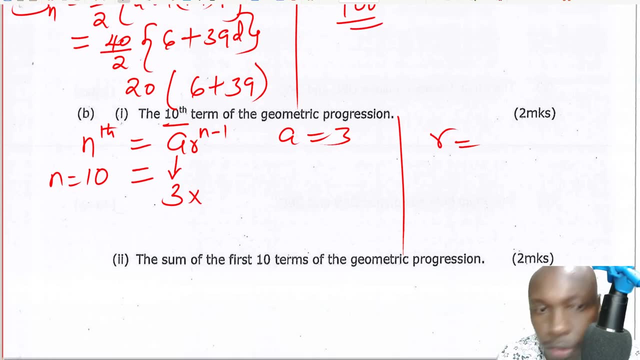 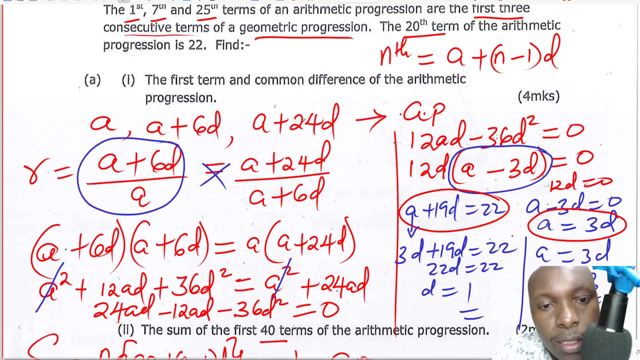 equals to substitute 3 times. uh, now the common ratio. we need to get the common ratio. don't have the common ratio, and to get the common ratio we just need to use a look at these. one of these: a plus 6d divided by a, or a plus 24d. 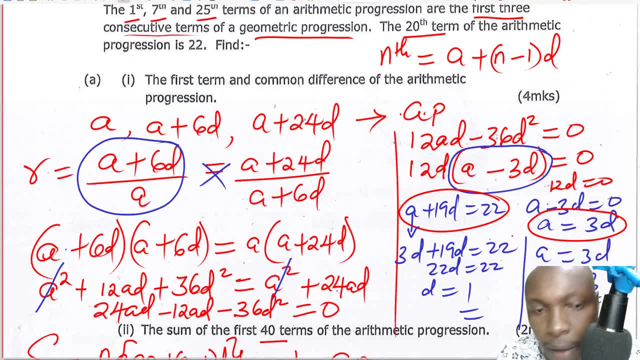 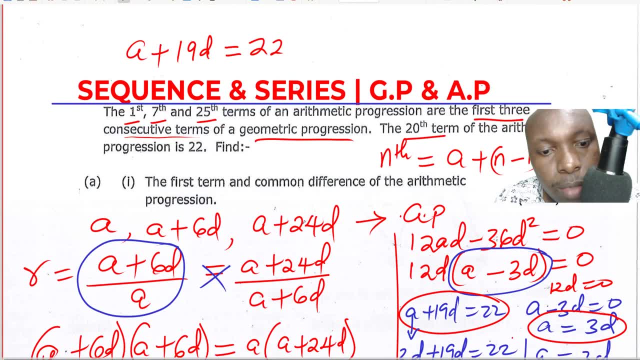 a plus 64d divided by a plus 6d. so i'll just pick this: a plus 6d, a plus 6d, a plus 6d divided by the rated by a. a plus 64d, a plus 64d divided by a or a divided by a to me: 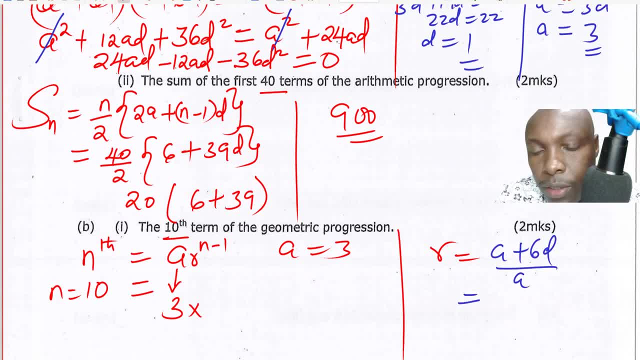 is four dummies divided by bay a, and this will give a is three, then d is one, then like not, so this will give 1 by 2, then d is one and then not, so this will give 1 by 2. 1xd divided by最低. 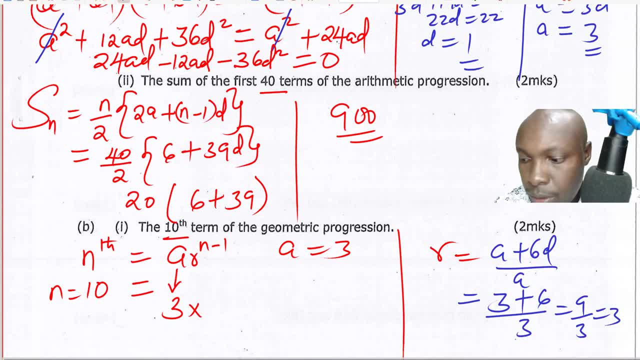 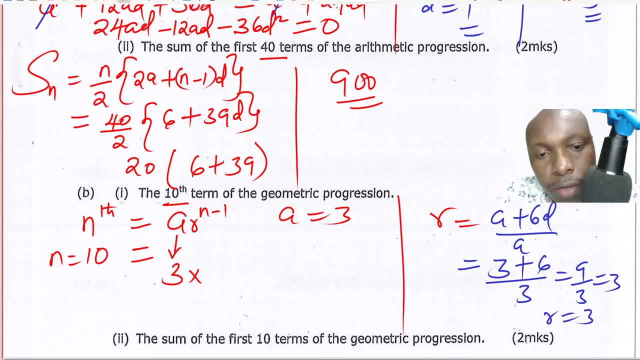 2xd divided by 3. so the common ratio is is three plus yes, it is okay, it is okay. r is three. so now substituting here is three, then r common ratio is three. then you have to raise the zone to the power of um. so raise the zone to n is 10 minus one. so this one will give three. multiply by three, raised power. 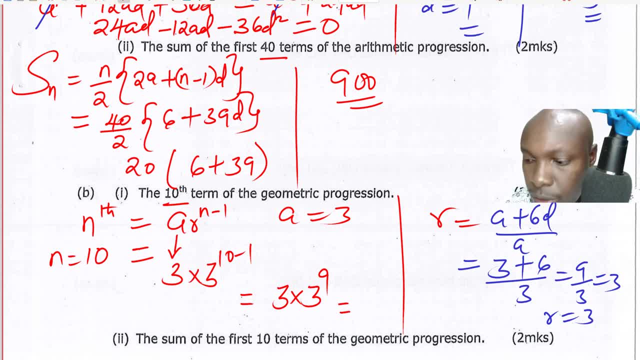 nine and that is uh what you get. after you work it out later you get um, you give a 59 000 and 49, 59 000 and 59. so by just having a is three, then common ratio, you obtain common ratio. here is three then n, if it is the tenth term, the tenth term and will be ten, just use these. 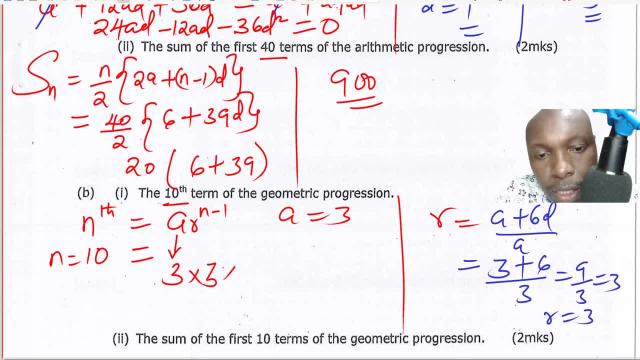 then r common ratio is 3, then you have to raise this one to the power of. so raise this one to n is 10 minus 1. so this one will give 3 multiplied by 3, raised to the power, 9, and that is what you get. 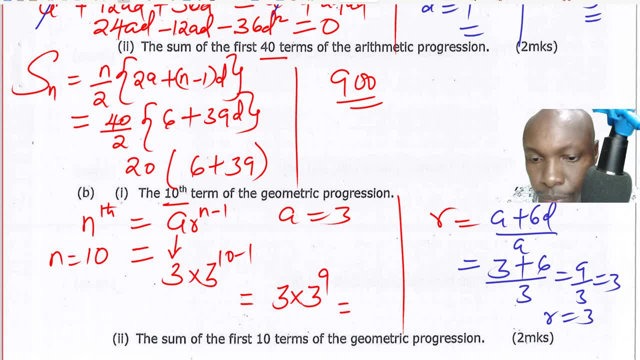 after you work it out later, you get um, um, um, um. this will give 59,049, 59,059. so by just having a is 3, then common ratio, you obtain common ratio. here is 3 then n if it is the 10th term. 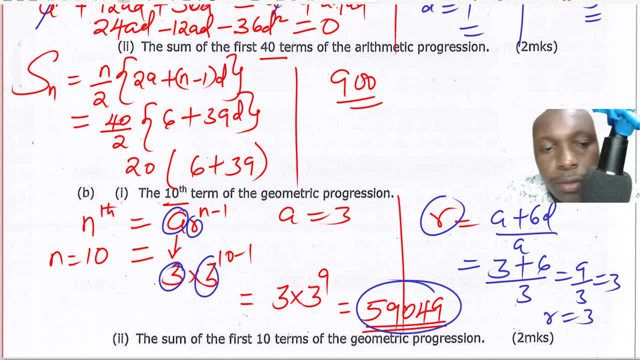 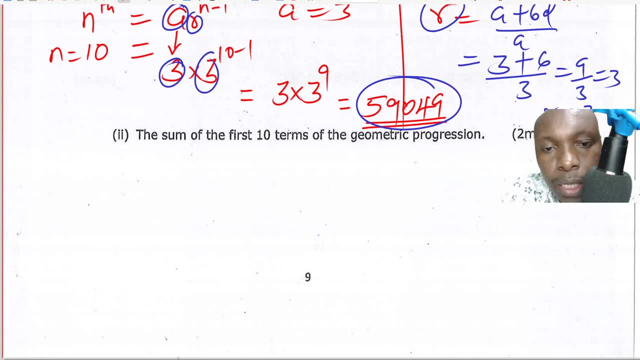 the 10th term, n will be 10. just use this, having the knowledge of the nth term now. then the other one is the sum of the first 10 terms of the gp. how do we get the sum of a number of terms, of any number of terms of gp? 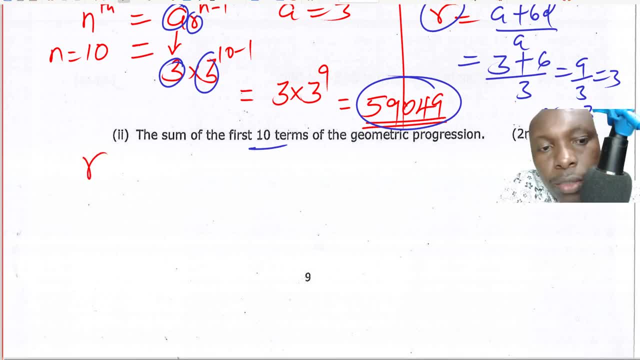 geometric progression. there are two formulas. one is when r is greater than 1, and the other one is when r is less than 1. now, in this case, r is um 3, so r is greater than 1. which formula is that the formula? this formula is in the four figure mathematical table. 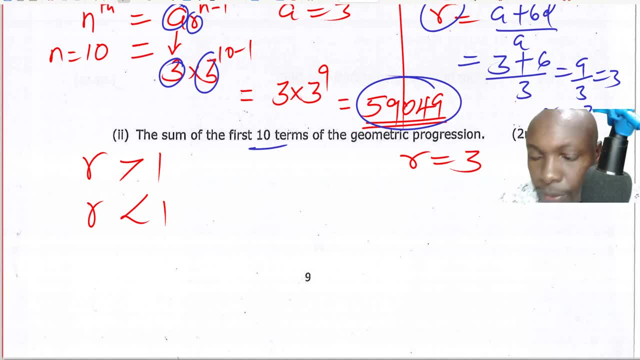 which you are required to use when you're doing your exams. we don't need to worry about this. so, given by s, n is equal to um. this is a. r is minus n minus 1 and r minus 1 just confirm this. so this is the formula when r is greater than 1. 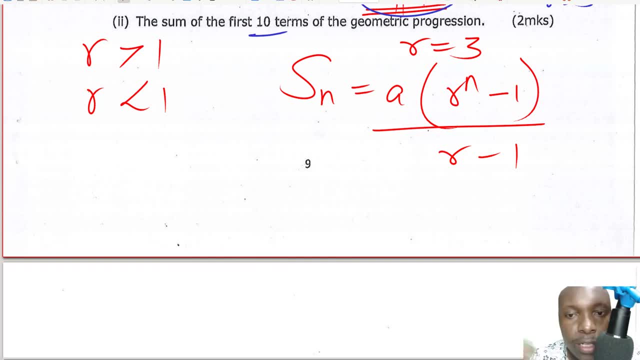 when it is less than 1. you know it's the formula to use. you don't need it at this time. so now, substituting this one: a is 3, then ratio, common ratio, is 3 as well. then, since the 10 terms, the first 10 terms, 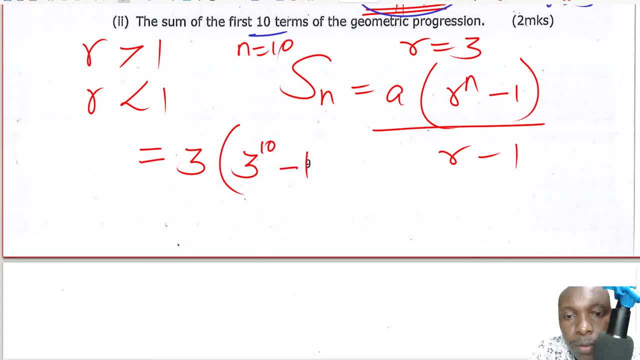 n will be 10, so 10 minus 1, then um r minus 1 will be 3 minus 1. uh, working out these? uh, you just need to use a calculator: 3 multiplied by the raised power, 10 minus 1, then 3 minus 1.